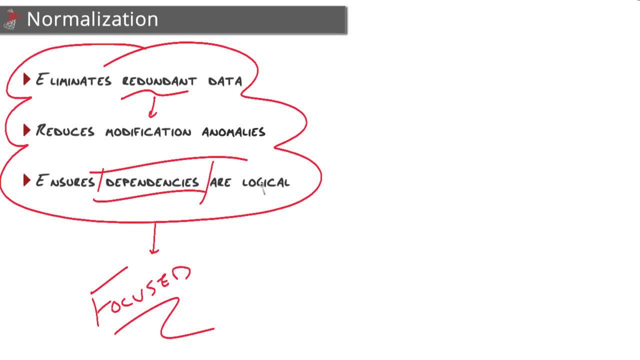 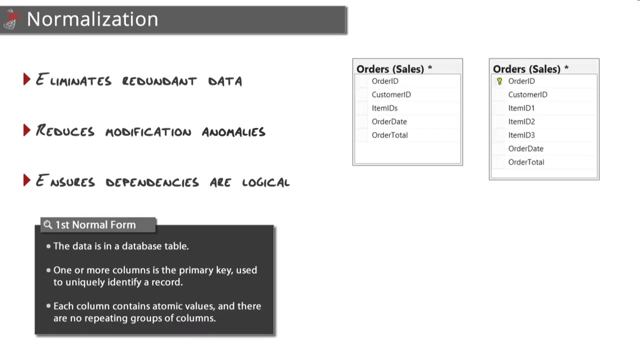 which can greatly simplify the queries that will be written down. As for the first normal form, here are the three requirements for first normal form. Number One: The data is in a database table. Where data is in a database table is a one table table. Number two: Mark your own data priority in order to Famobu and use the same bad direction. Next one is normalize your short file design. Number three: normalize your form without causing major problems, asule matters like time optimization. Number four: normalize your long file rules. 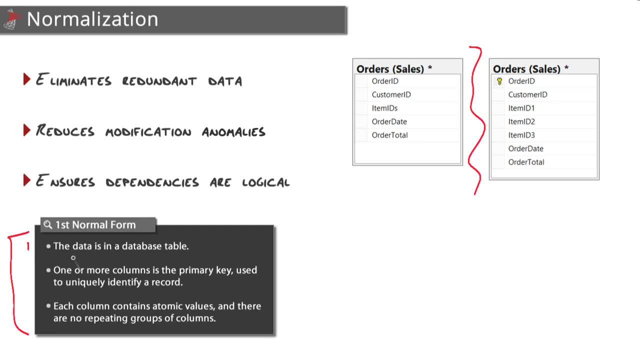 Say: don't manipulate yourپkpn, but avoid cheating benches. This doesn't look like a laughing다나. Hallvuhdz improvement, we're good there, But I will mention that it does help to actually look at data so you can visually. 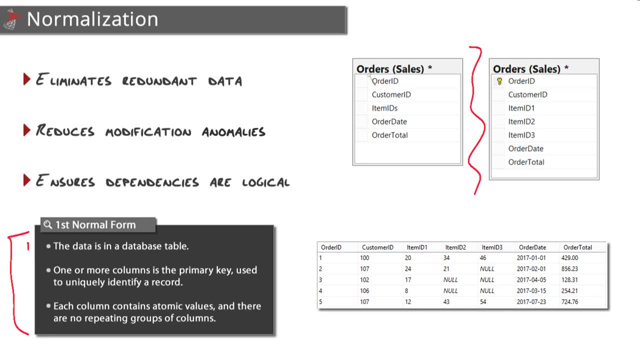 see some of the problems that you may not initially see by looking at the design of a table. And if you're trying to improve the design of an existing database by sending it through normalization, that's pretty easy because you'll probably have data to look at. But if you're working with a 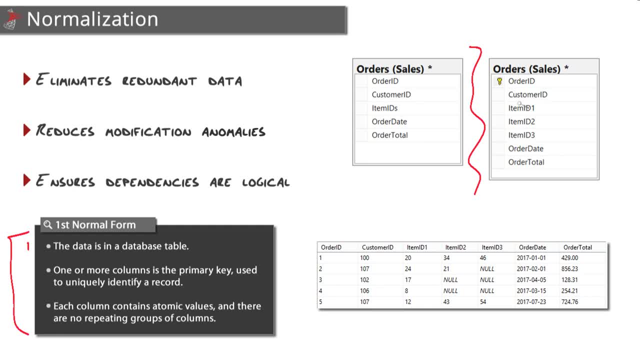 new design. you probably won't have any data inside of it, And that's where you can go out- and there's all kinds of data generators out there- and fill it up with just dummy data And that way again you can eyeball it to see: oh look, there's redundant data all over the place. 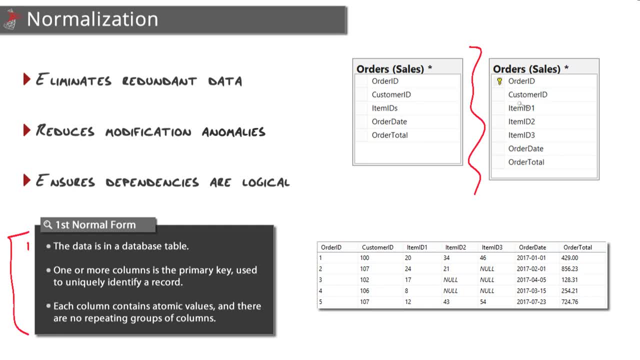 or look, there's a cluster of null values And that'll help you get a little insight there when visually attempting normalization. So just a little side note there. but we're good, Our data is in a database table. Number two, one or more columns is the primary key used to. 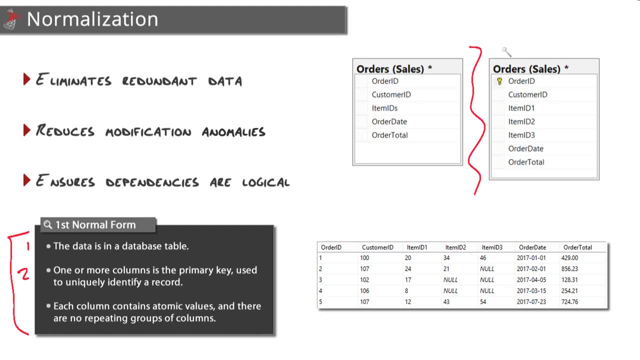 uniquely identify a record. Our second table is good there. right, We meet that. we have a primary key on order ID. Our first table does not. We do not have a primary key, so we would need to put one right there. The third one is the big one. here. for first normal form, Each column contains: 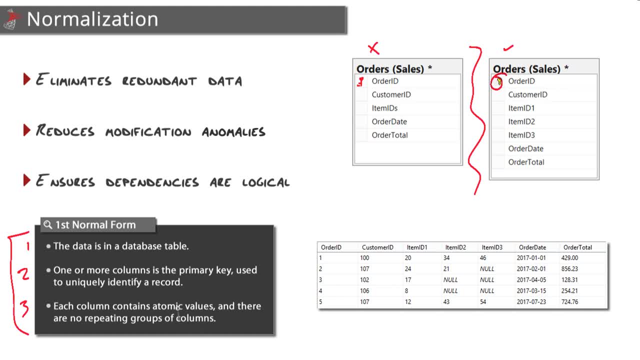 atomic values, meaning the value cannot further be broken down and there are no repeating groups of columns. Both of these violate this third rule here. Our first table has an item IDs column, which you could think of as item IDs, separated by a delimiter like a comma or a semicolon. 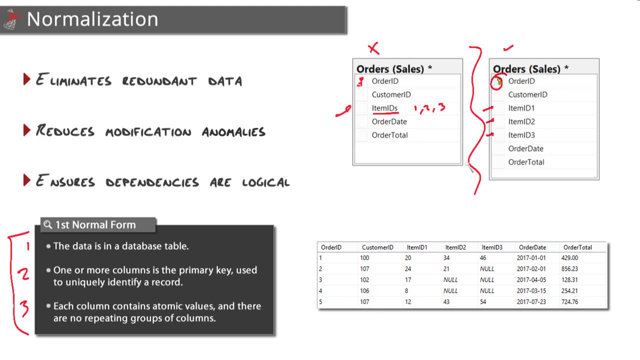 Our second one violates it because we have a repeating group of columns: item ID1,, 2, and 3. This is poor design because we're going to have a lot of null values if we're only selling one item. And what if we need a fourth or fifth or sixth item? We're in trouble. 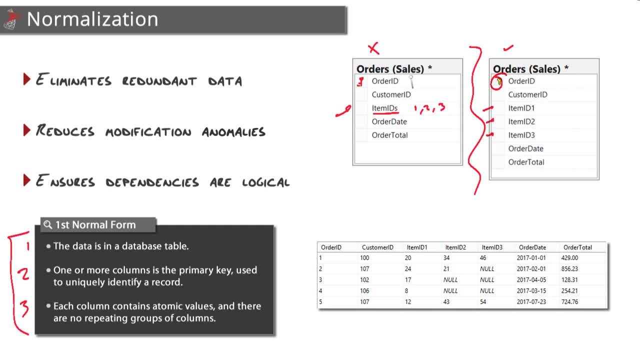 here. This design does not lend itself to that. So the root cause of this problem is that when a customer makes an order, they can order X number of items, And we're trying to represent that relationship within the orders table itself, which isn't going to work. A proper solution here. 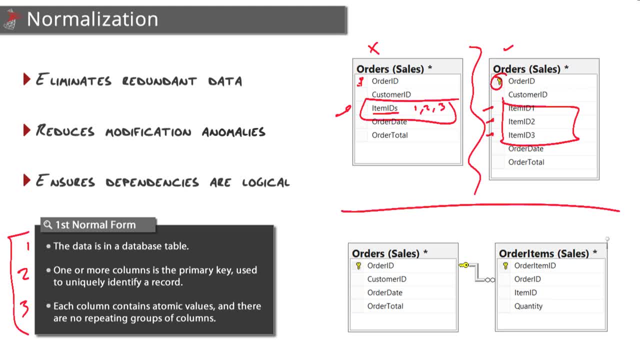 would be to break that out into its own separate table. So now we have essentially an order table and we're going to be able to break that out into its own separate table. So now we have essentially an order table and we're going to be able to break that out into its own separate table. 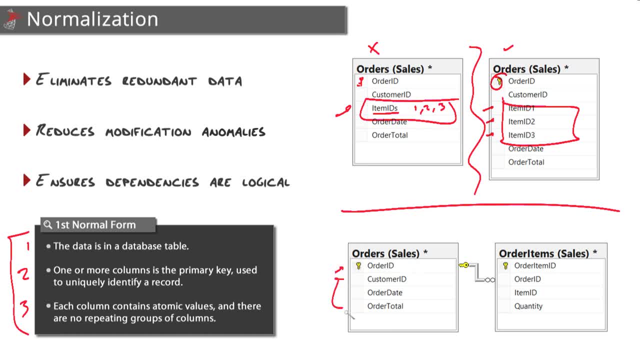 So now we have essentially an order header table that contains information just about the order itself and the customer who ordered it, And then we have an order items table that will contain a record for every single item, line item- on that order, And that's why we have a one-to-many. 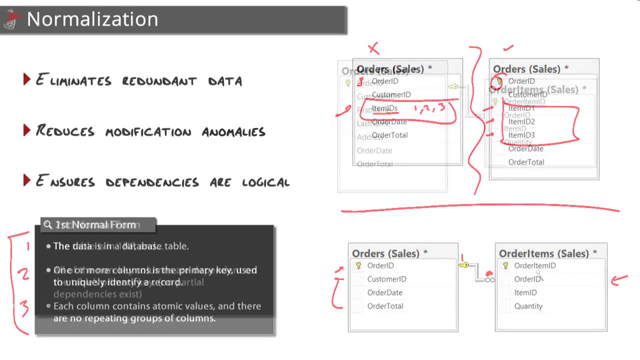 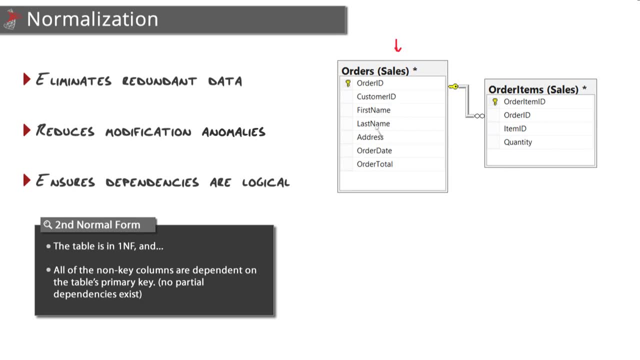 relationship here between an order and the order items. Moving on, let's look at second normal form. Now let's take our orders table once again and let's say we need more information about the customer. So we added first name, last name and address into our orders table. Now there's two. 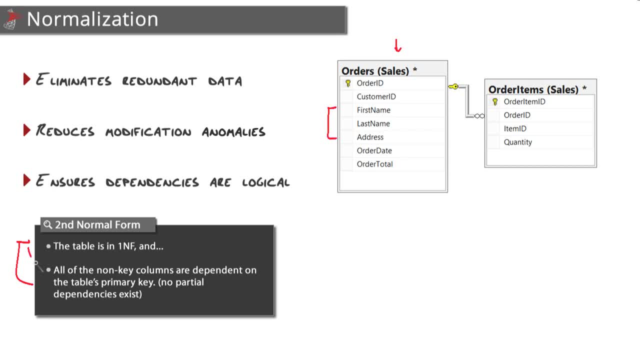 rules for setting up an order table. First, we're going to be able to set up an order table. second, normal form. The first one is that the table is in first normal form. Is it? Let's find out here. Do we have a primary key? We do so. we're good there. Do we have any repeating groups of? 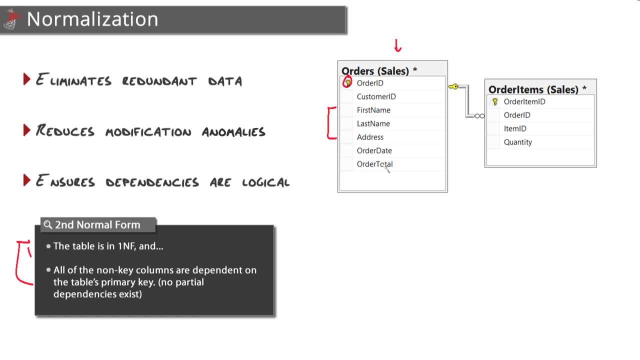 columns. Nope, we're good there. And each one of these columns contains atomic values. Good, so we're good there. What if we just created a customer name rather than first name and last name? Would that have been atomic? No, it wouldn't have been, because it just would have been name. So we broke. 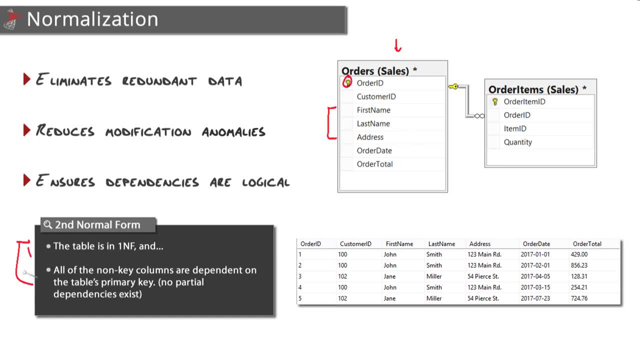 that down into first name and last name? and yes, this meets first normal form. What about the second one? here? All of the non-key columns are dependent on the table's primary key. In other words, we can have no partial dependencies. Let's test it out. What about customer ID? Does that depend on the primary? 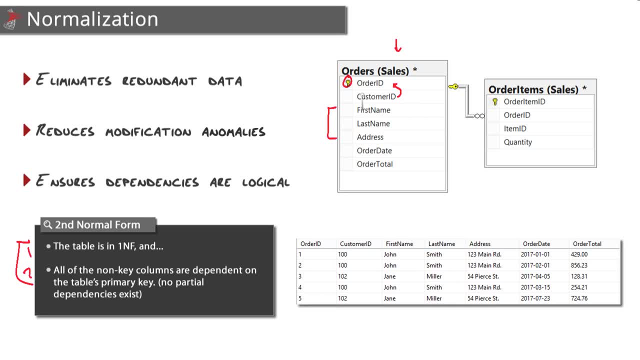 key. This is an orders table, so an order is placed by a customer. So, yes, customer ID absolutely depends on the order ID. What about these next three: first name, last name, address- Do they depend on that order ID? No, they depend on the customer ID right. First name, last name. 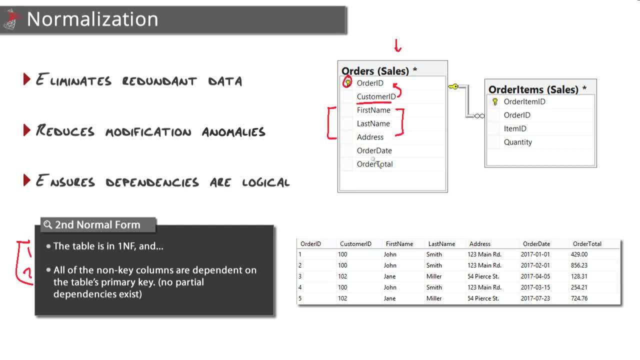 address are tied. The order ID is tied to the customer, not the order. So these three fields columns do not belong in this table. What about order date? Yep, that's good. That describes the date that the order was placed. And what about order total? Absolutely, that also describes the amount of this order. 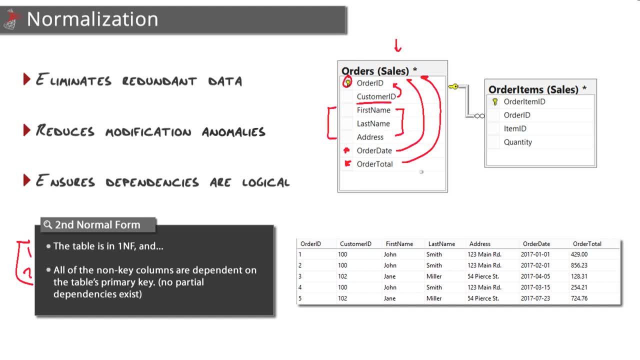 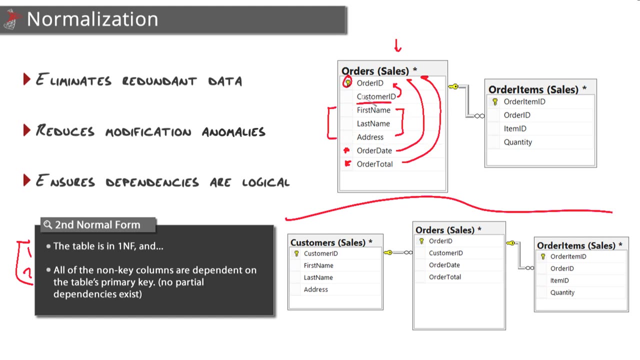 This is another area where seeing the actual data can really help you identify problems with tables that aren't in second normal form, because you will see a lot of redundant data in those columns that don't depend on the primary key. And, by the way, here is the solution: Again, we take those columns, those columns that are: 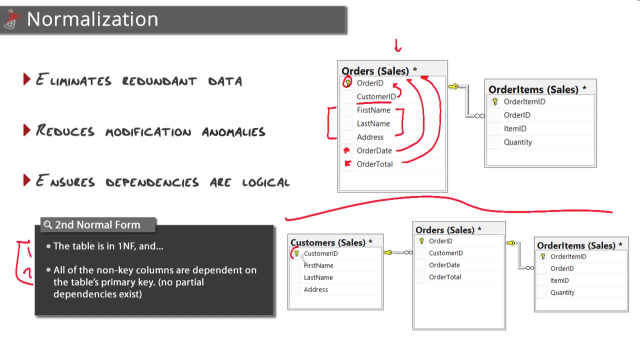 redundant and place them into their own table. So here we should have a customer's table with the customer ID as the primary key, linked to that customer ID, which will be the foreign key in that order's table. So you can see, the process is really just breaking things down. 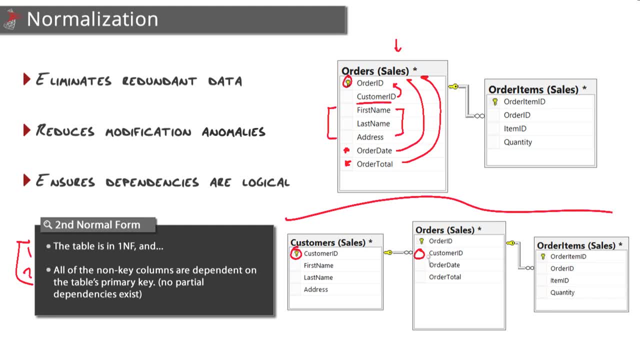 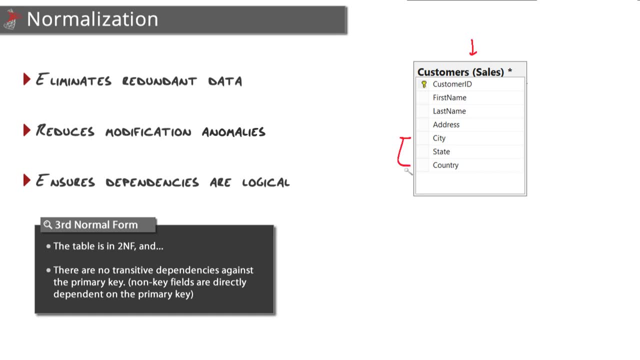 creating more tables that are all focused on containing just their data elements. Moving on to third normal form, let's take our customer's table and say that we wanted to add a table to our table, And we can see that we have a table that comes into here to track exactly. 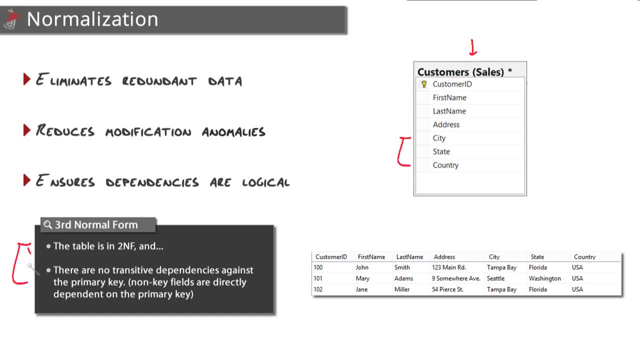 where customers live so we could deliver them our products. Here are the two rules for third normal form. Again, the first one is that the table is in second normal form, which it is for the most part. One could argue that city should actually probably have a city's table linked through city ID, which 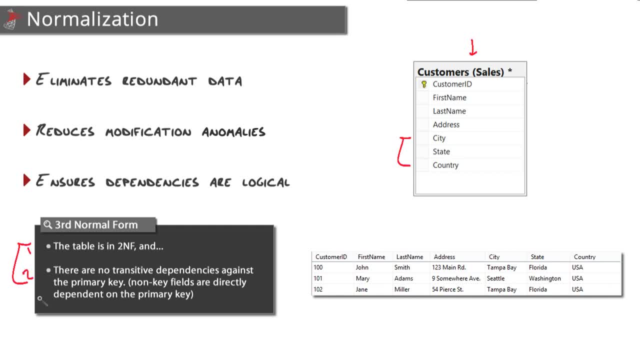 we'll do here in a second. But the second rule here is the big one: that there are no transitive functional dependencies against the primary key. And you're probably asking yourself what the heck is a transitive dependency. Think of it as something that depends on something through. 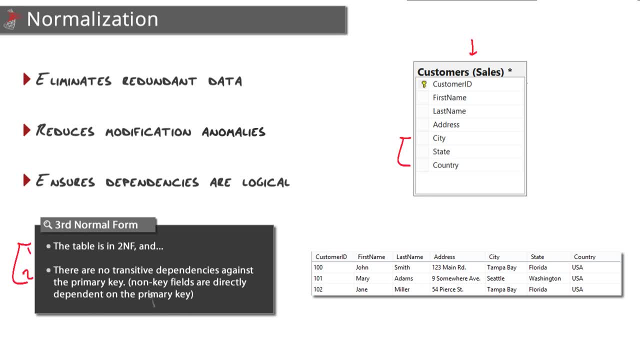 something else, And that's why I put in parentheses here. non-key fields are directly dependent on the primary key. So once again, you want to go through each one of these columns that you've defined and ask yourself: does that depend on the primary key? First name, last name, address, city, they all. 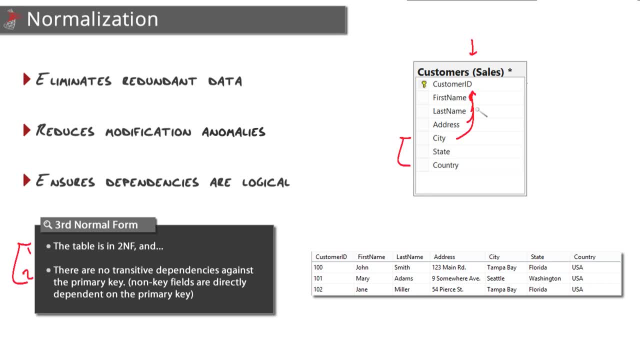 depend on that customer. They describe exactly where that customer lives. State, however, has a transitive dependency on customer ID through the city And country through the state which state through the city. So these last two here are transitively dependent. 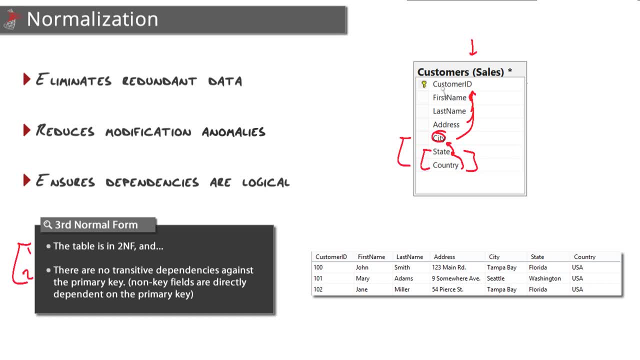 on the customer ID. The city already describes where the customer lives, but the state requires the city and the country requires the state. So that's why these two should not belong inside of this customer's table. So a better way to describe this would be to break each one of those dependencies. 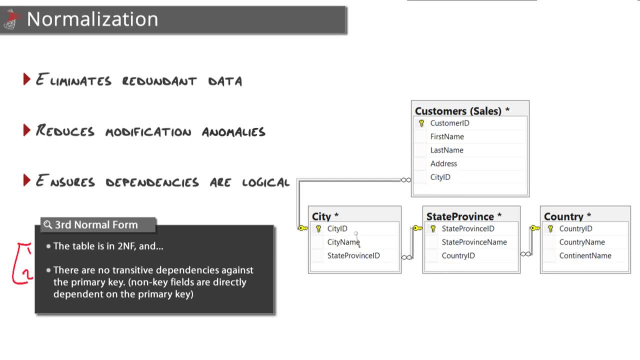 off into their own table. So now we can link the city table through the city ID, the state to the city table and the country to the state table And again the effect that this will have is dramatically reducing the amount of redundant data that we would have had in our previous customer table design. So you can see the 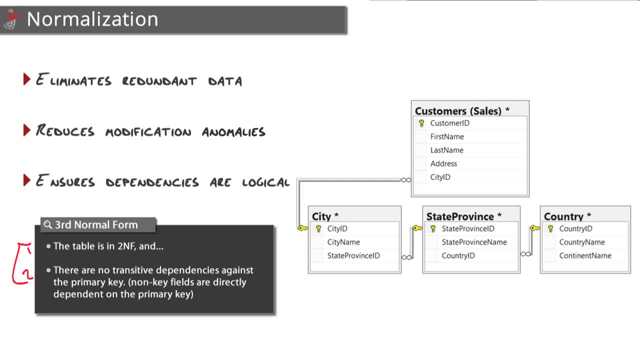 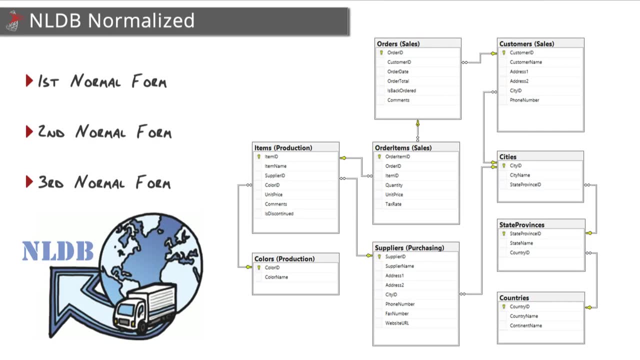 whole process of normalization is just continuing to break things down as far as you can go, until every single table is its own focused entity. And here's the final logical design of our NLDB database, taken down to the third normal form. So those three tables that we 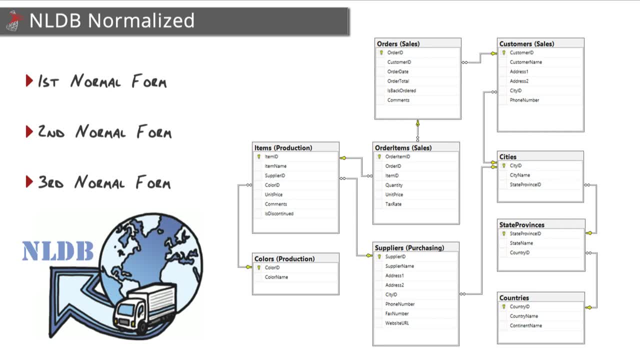 looked at in a previous nugget, have really been broken down here into many more tables. So most of these we've gone through in this nugget. but I just want to point out here that we took color name and put that into its own table to reduce the amount of redundancy there with colors And same. 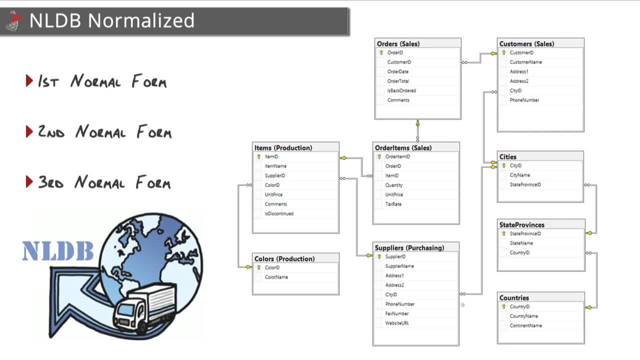 with suppliers. We did just have supplier name, but we also broke that into its own table, which also gives us an opportunity to track more information about our suppliers, And that's that We are now ready to transform this into a physical database. In this CBC Nugget we talked about the benefits. 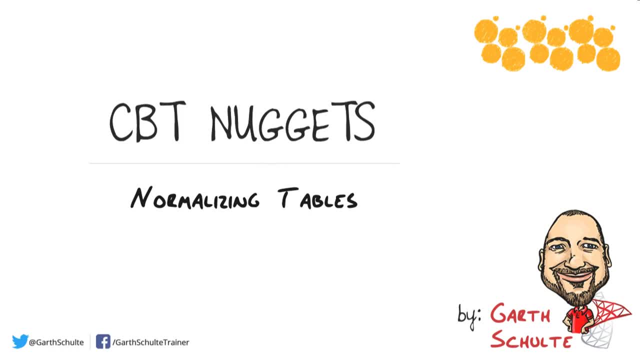 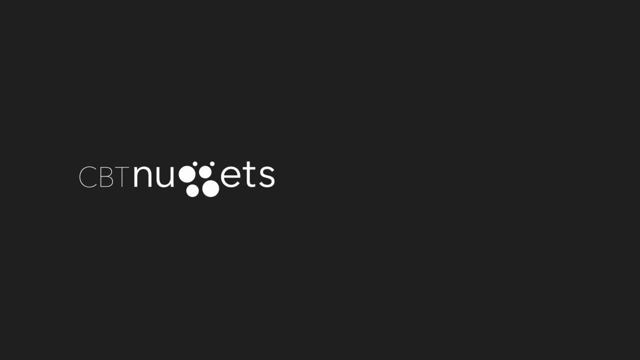 that normalization provides to our database designs and also how to take a table and send it through the first three normal forms. I hope this has been informative for you and I'd like to thank you for viewing.